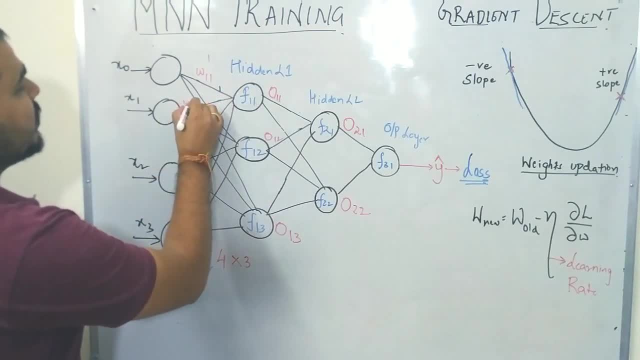 Now, similarly, if I want to specify for this, this can be specified as w21 hash. That basically means that from the second neuron the input feature is getting supplied to the first neuron of the hidden layer, And similarly we can draw: 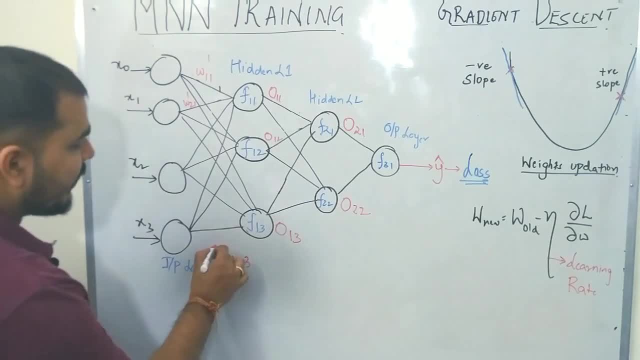 Whereas this is theamı with respect to a particular seb新 lawyers. Different types of weight, we can mention it over Here, But the matrix of the weight will be four X three. This will be 4 X three A matrix and with respect to this particular for cross, the matrix in my next layer. 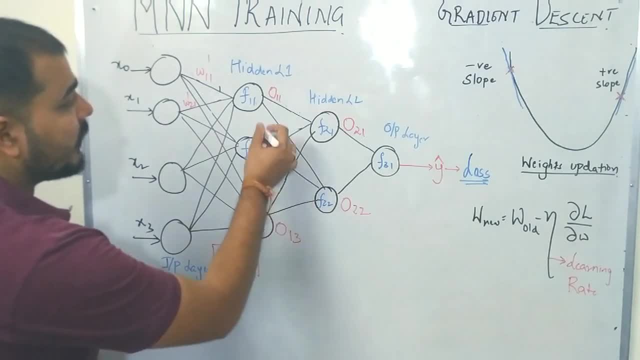 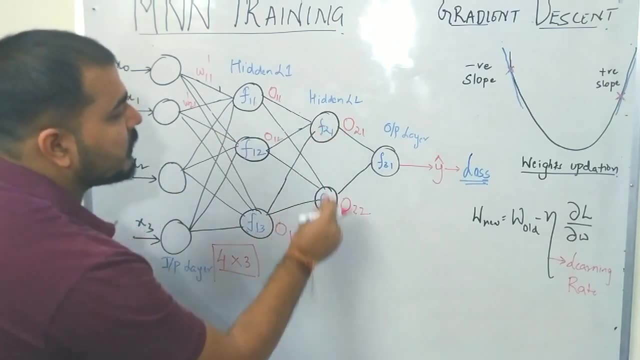 Whenever I go to my next layer, Then this will basically I will be having three outputs from here There. So this matrix will be three cross. I have two neurons Hidden layer in the two, so this will become three cross two. 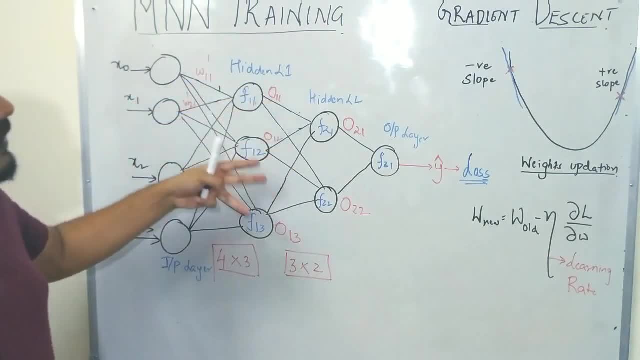 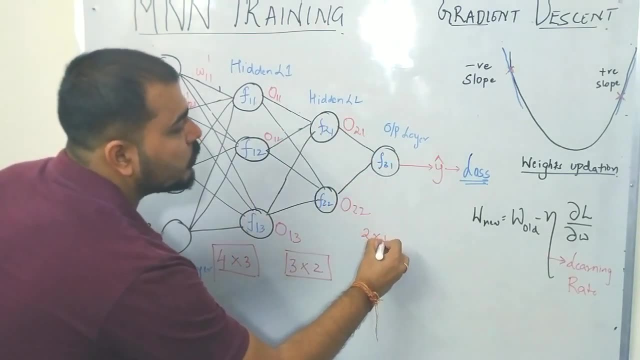 Mattricks, You know that basically means that we have To specific Exact With three weights with respect to two hidden neurons and similarly, finally, when we go to this particular output. this will basically become two cross, one matrix of weights and the inputs. Now, as you know, 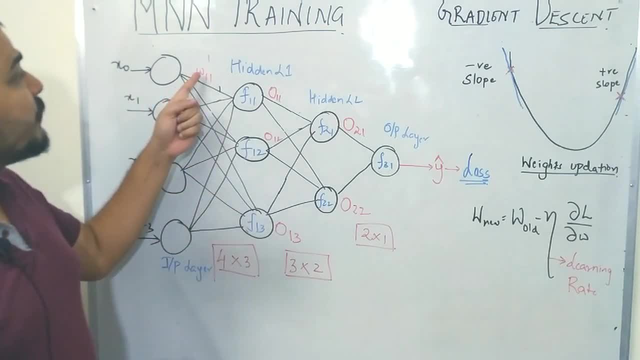 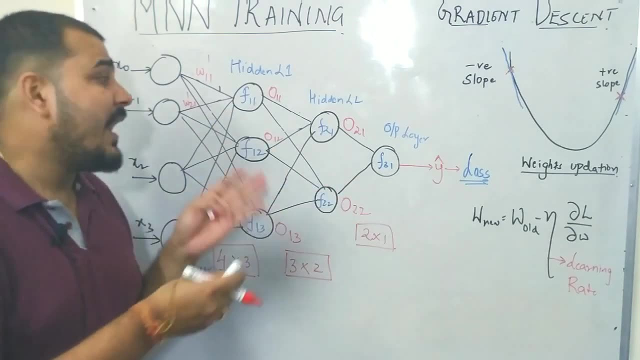 that what happens in the hidden neuron, in the hidden layer. this weights will get multiplied right with the input feature and all the summation will happen and a bias will added and then an activation function will get applied. The activation function can be sigmoid and relu. I still have to. 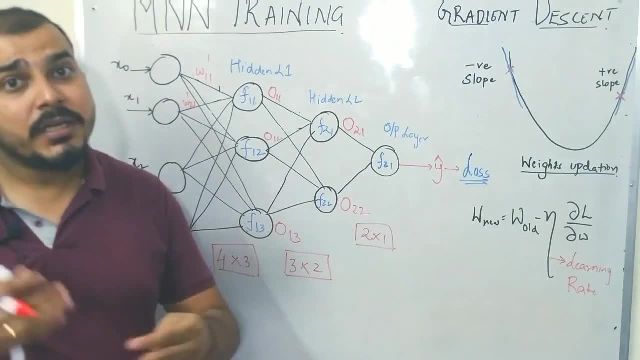 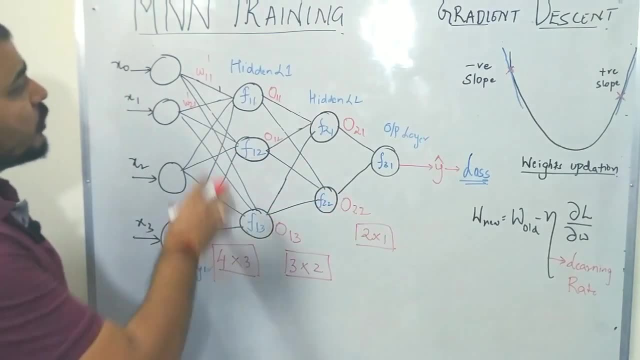 discuss about activation functions and that I will do it in my future classes. but you need to understand first this and then we will try to understand when to use what kind of activation functions. So this kind of operations takes place in each and every hidden neuron. Then what will? 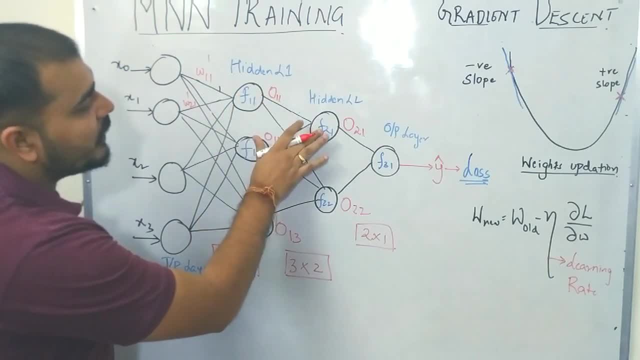 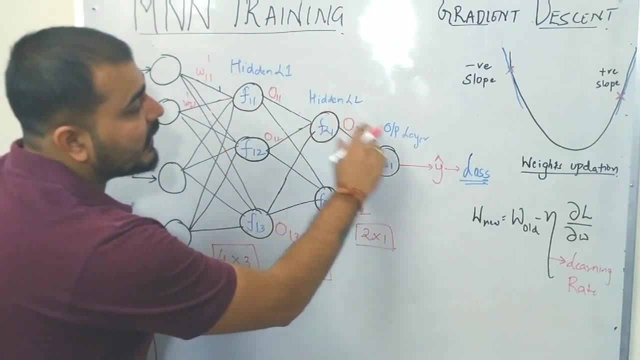 happen, then again this particular weights will get assigned to this particular layer when the input, when the output get supplied from the hidden layer 1 to the hidden layer 2.. Similarly, finally we will get this particular output layer and finally we will get y hat, which is my y predicted. 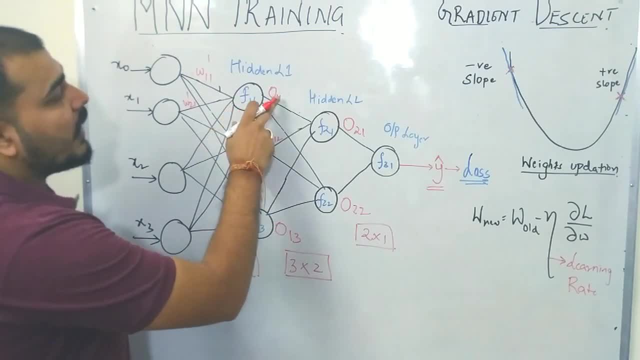 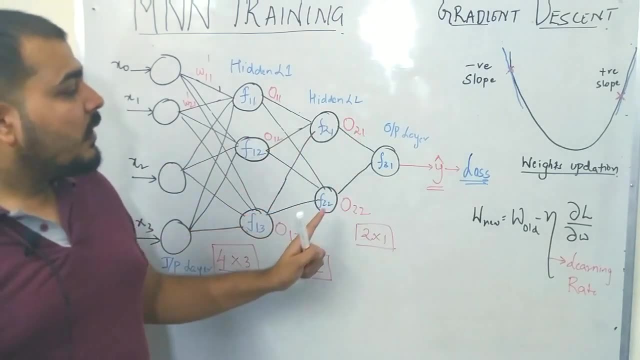 result. Now understand guys. the output of f double 1, I have written as 0, 1, 1. the output of f 1, 2, I have written as 0, 1, 2.. Similarly, the output of f 2, 1, I have written as 0, 2, 1, and output of this f 2, 2 is. 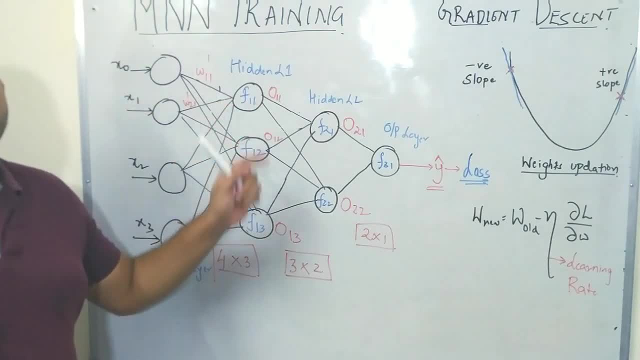 basically written as 0, 2, 2.. Why I have written this function? This function does two kinds of operation, as I have already specified before. First of all, all the inputs will get multiplied with the weights. the summation will be done, a bias will be getting added, and after that this: 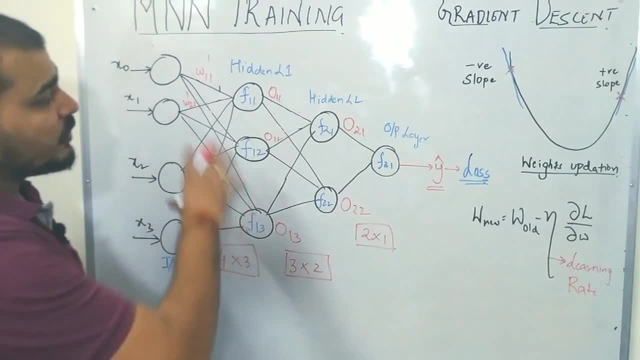 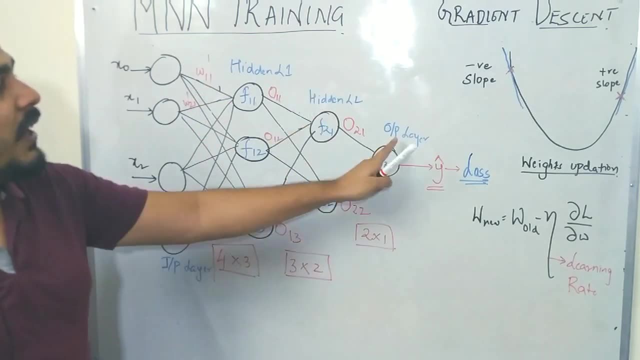 functions will apply an activation function on top of it. Okay, so that is why I have just written f 1, 1, f 1, 2 with respect to the first hidden layer, Then second hidden layer, I have written f 2, 1, f 2, 2 and finally, my output layer, I have written as f 3, 1 and now I 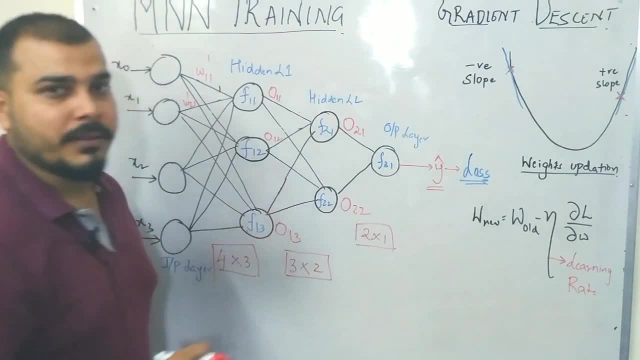 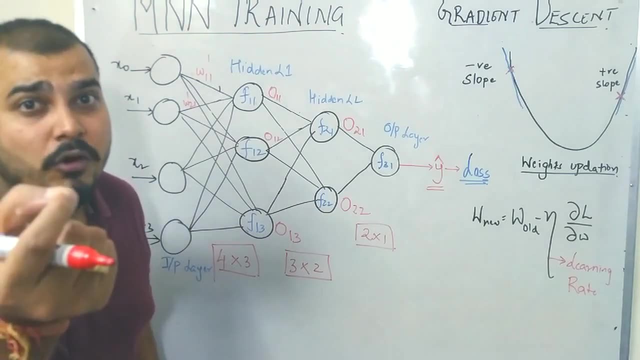 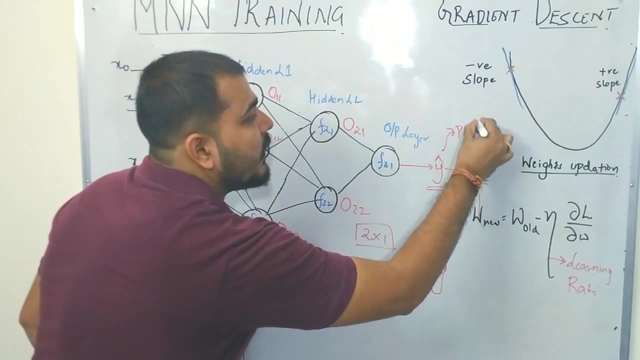 am getting my output. that is my predicted value. Now, what will happen now? what will happen now? just imagine that this is my input features. with respect to my input features in my training data set, I will be having 1 output. So this y hat is basically my predicted value. predicted value. 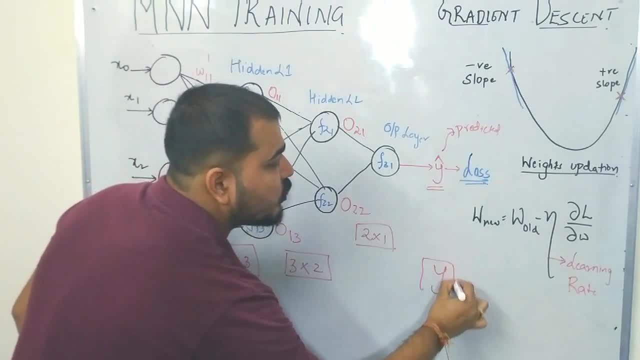 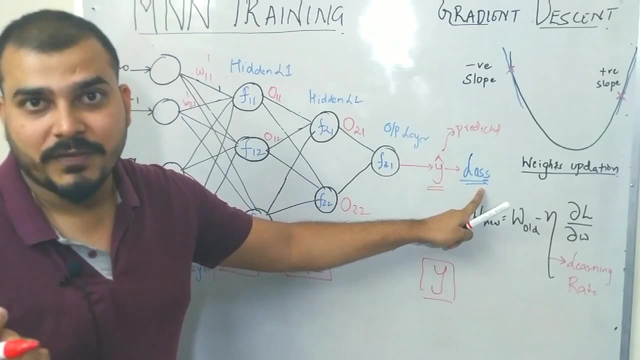 right, Right, Ok, And then y will actually be my actual value. Now, this, too, has to be getting compared. right For that, what do we use? We use something called as loss function. okay, We use something called as loss function. 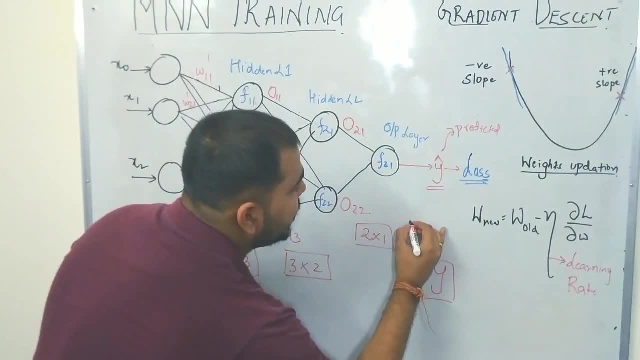 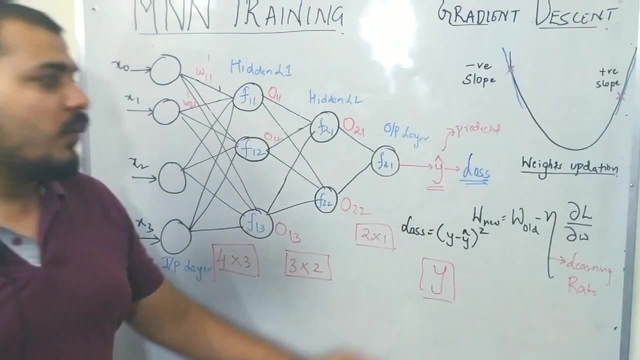 Now loss function can be defined something like this: So here I will just write down my loss function. It will be y minus y hat whole square, right, y minus y hat whole square. That basically means I am trying to see the difference between y and y hat. 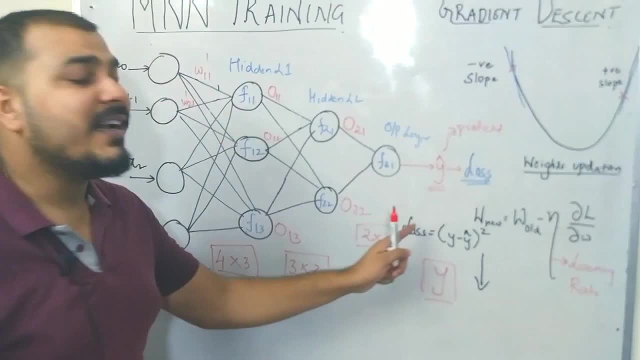 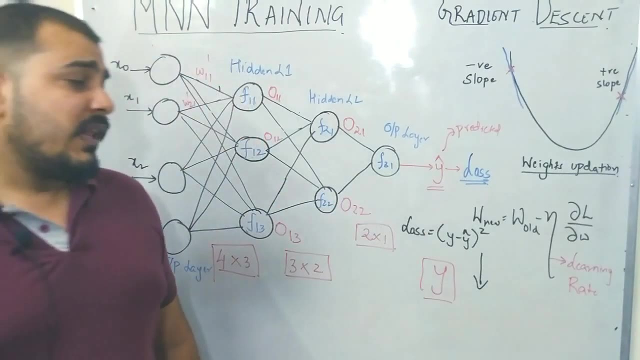 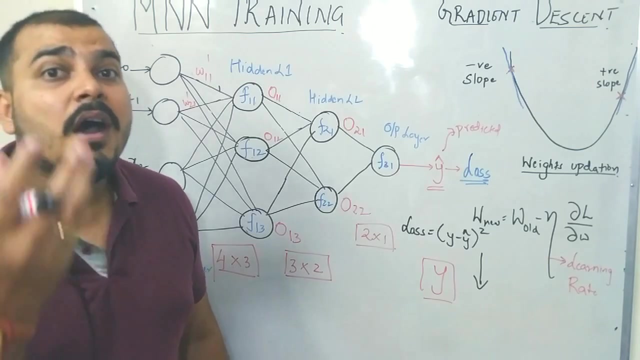 And my main aim is to reduce this loss value, Then only I will be basically getting- I will be getting- the similar results of y, hat and y. Now I told you in my previous class, in our previous session, that if you want to reduce this loss function, we basically use an optimizer. 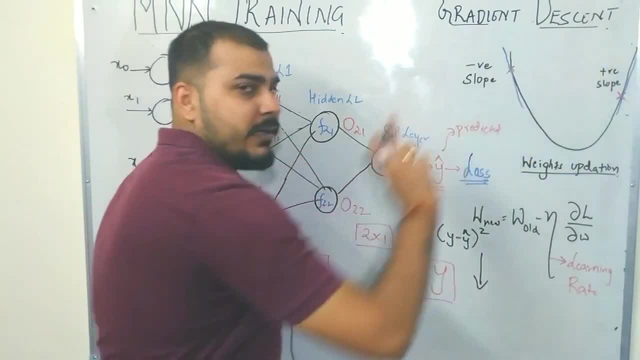 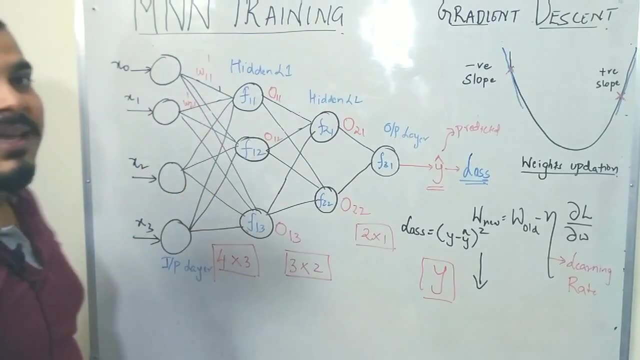 One of the example of an optimizer is something called as gradient descent. okay, Now, gradient descent work is to update the weights, update all these weights, In such a way- okay, In such a way- that we should be able to get y hat, which should be similar to y hat. 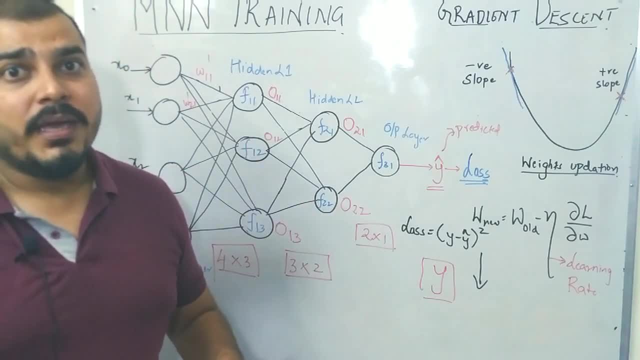 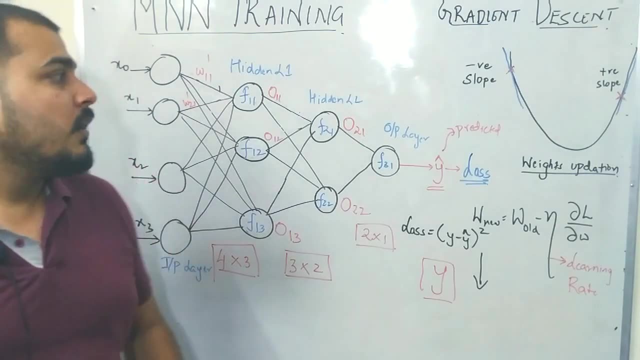 And that is what is the main aim of an optimizer. okay, Now, in this case, is gradient descent, Suppose. I am taking the example of gradient descent. There are other types of optimizer, like stochastic gradient descent and many more, But today we will just understand what this gradient descent does. 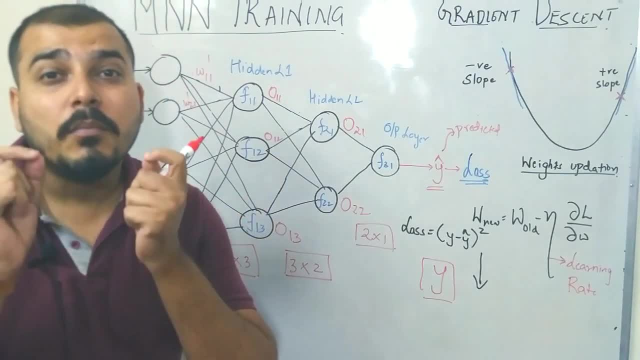 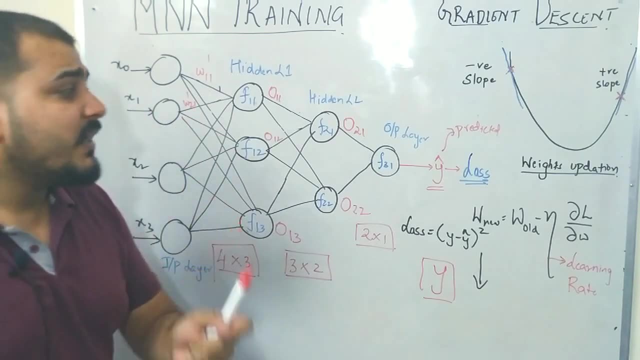 In short, gradient descent will try to find out the most. you know the weights. that has to be updated In a very efficient way and the best weights to calculate your y hat. okay, And that basically means we are updating this weights. 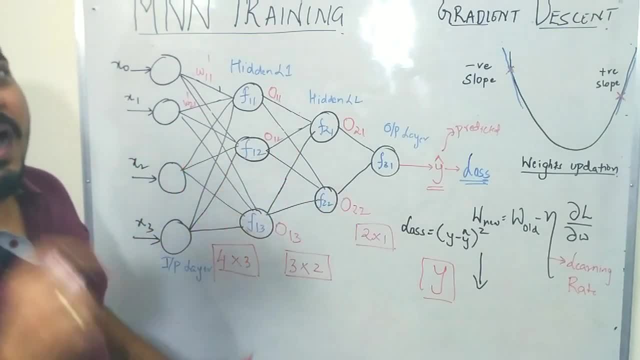 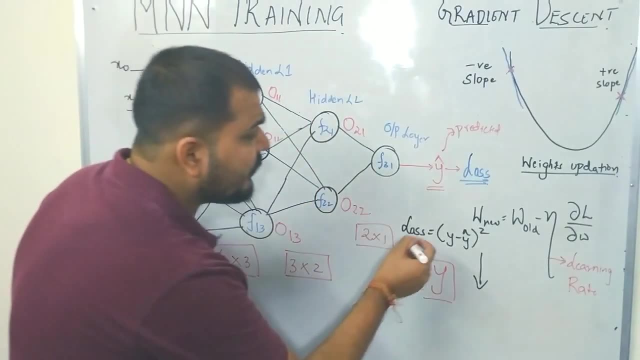 all the weights in each and every layer. okay, Each and every layer. how it is done, that process is basically called as back propagation. Now suppose, just imagine in the first back propagation what will happen. okay, Now I have got this particular loss value. 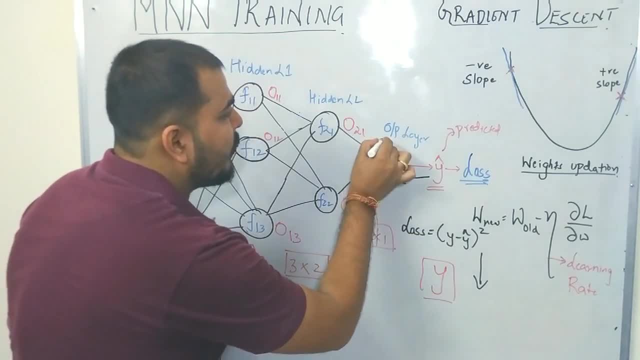 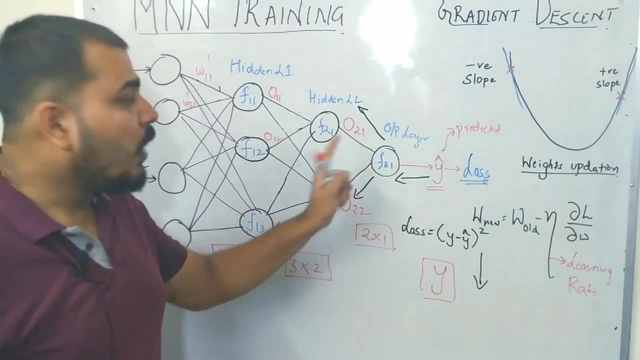 Now I have to back, propagate from here. right Now, when I back or propagate over here, I have to update this weights. I have to update this weights Because there are two weights over here. I have to update that. How to update this particular weights? 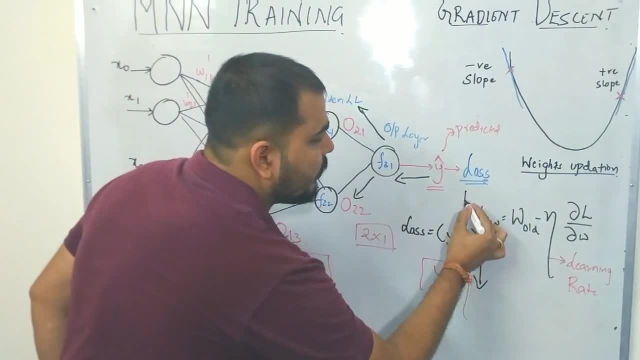 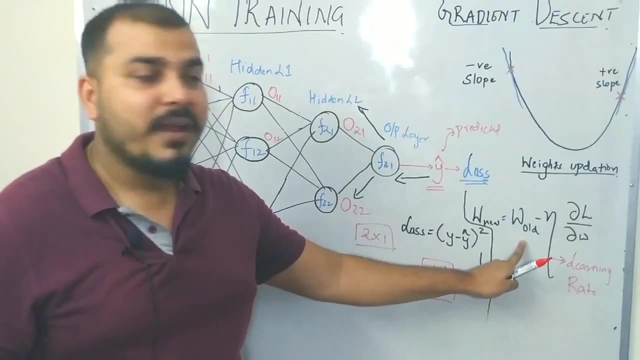 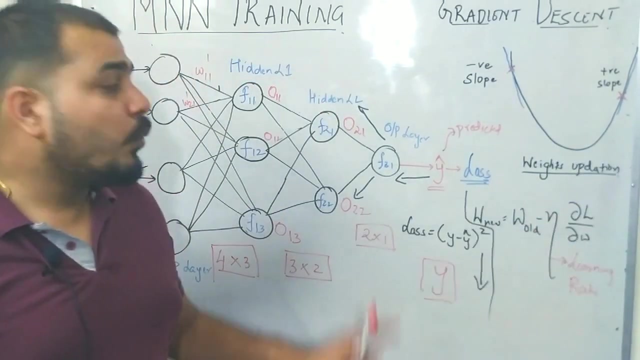 That we need to understand. So weight updation formula is something like this: okay, So here I have written the weights. the new weight will be equal to the older weight, minus learning rate, multiplied by derivative of loss divided by the weight itself. okay, 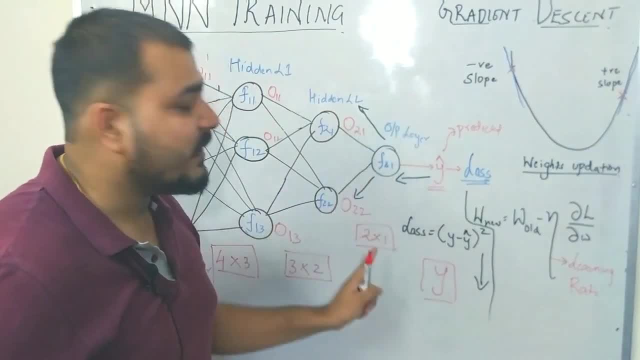 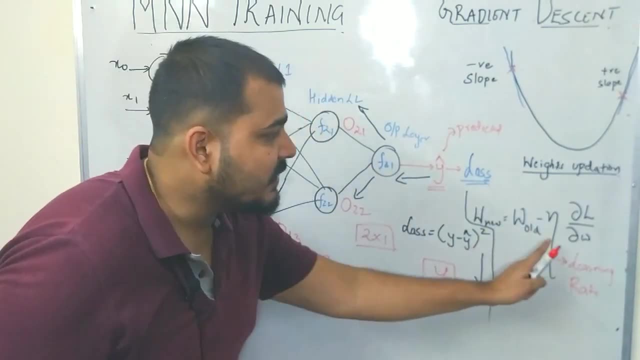 Derivative of the loss with respect to the weights of that specific weight. okay, Okay Again. I am telling you again, I will just repeat it: It is basically y, the older value minus learning rate, multiplied by the derivative of loss. 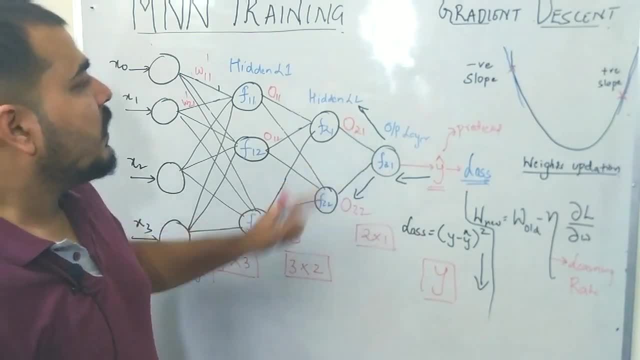 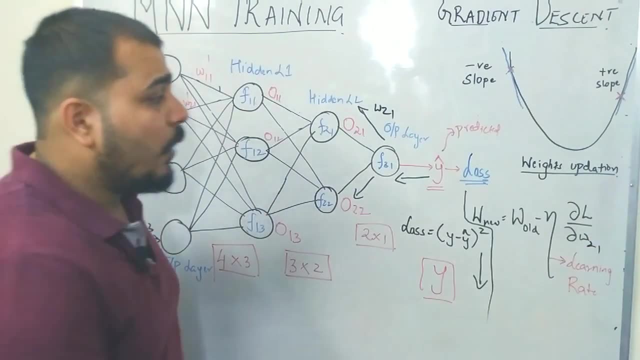 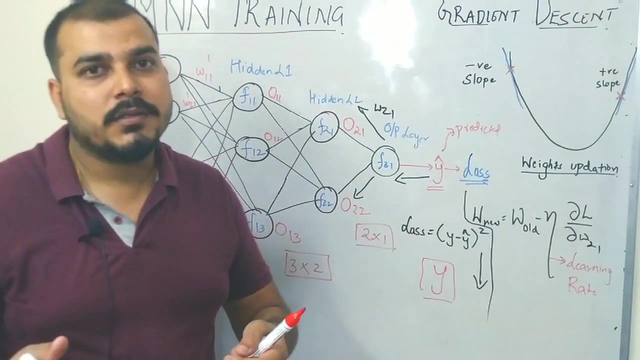 with respect to that specific weight. okay, In this case, suppose the weight here is mentioned as W21.. So this DW will may change to W21,. okay, Now why do we find out derivative Guys? if you remember in your high school days or if you have, if you are, when you are basically in 11th and 12th? 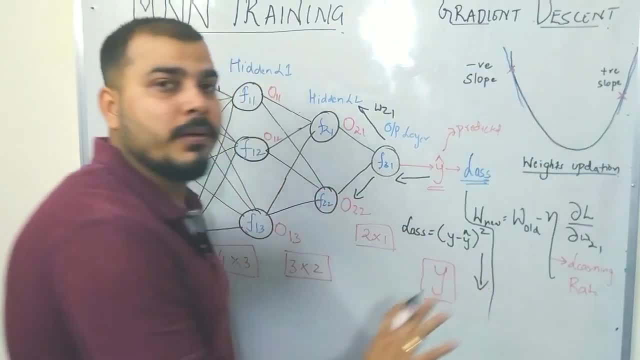 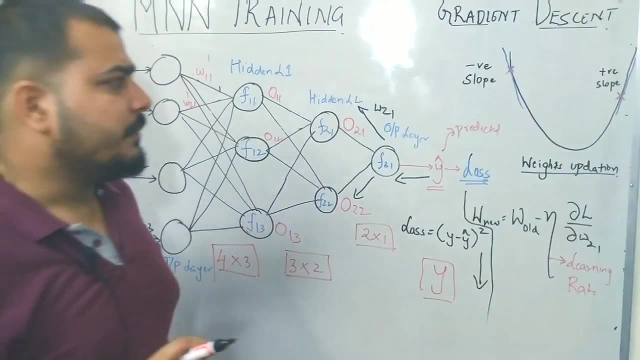 right derivative basically means we need to find out the slope. okay, Slope is basically the tangent line where we draw. what is the slope of this particular point? okay, Now just imagine- let me just consider- my initial weights were initialized to this particular point. okay, 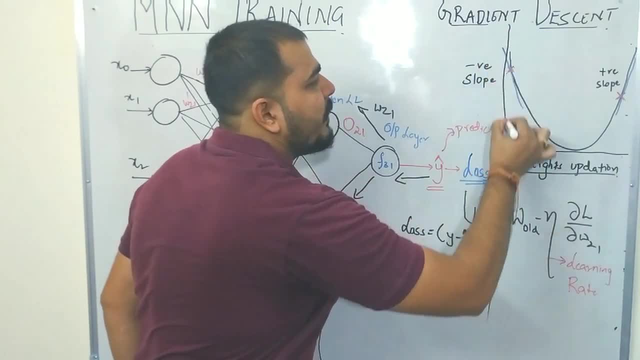 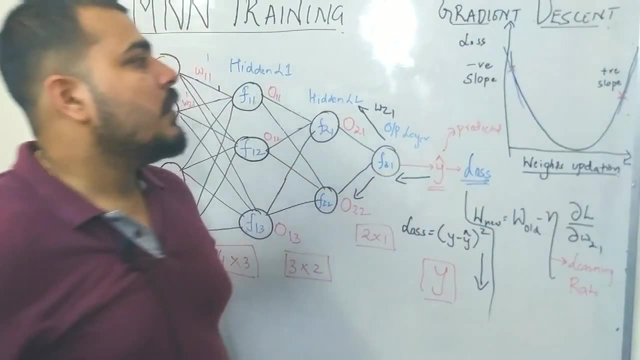 This point may be something like this: okay, This may be based on my cost function. okay, This cost function or the loss function that I have. okay, with respect to my weights. Now suppose my initial weights were pointed somewhere over here. okay, 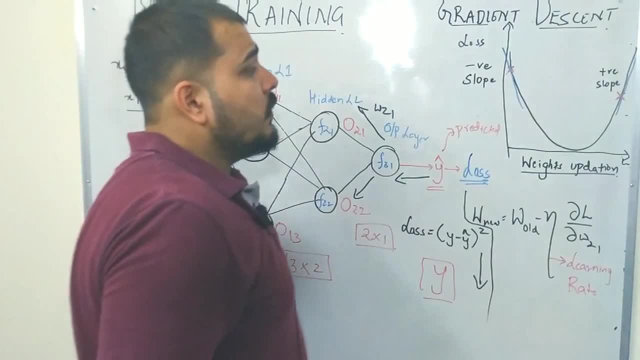 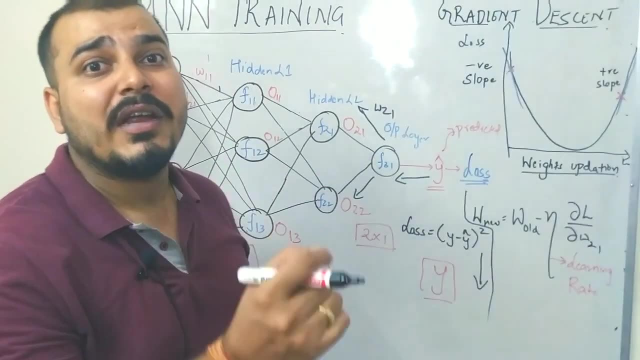 Initially, I have a cost function. okay, Initially, it was initialized over here. okay, Now, this derivative will help us to find out whether this, whether this slope that we are trying to find out, is positive or negative. okay, Now, in this case, in this case, I will say it as negative slope. 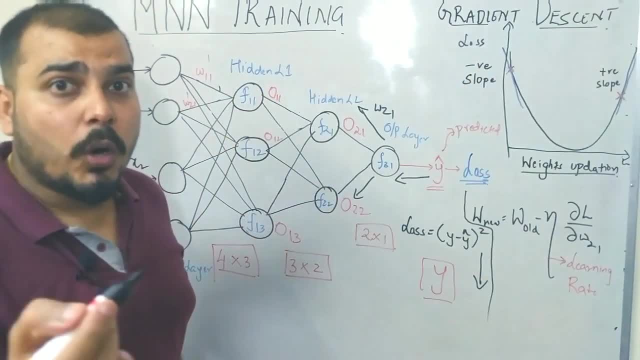 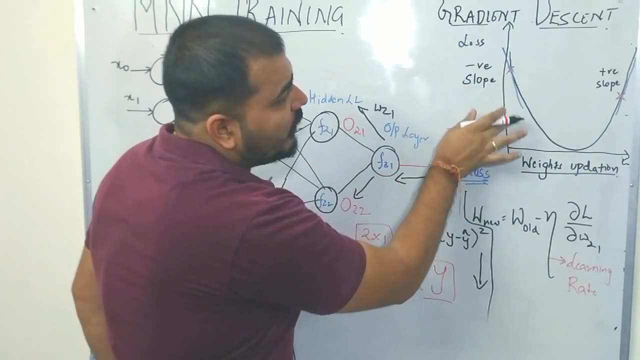 Why? Now, in order to find out slope or derivative, you will just draw a straight line passing through this particular point. okay, Then you see that right-hand side of this particular line, whether it is down or whether it is pointing up. 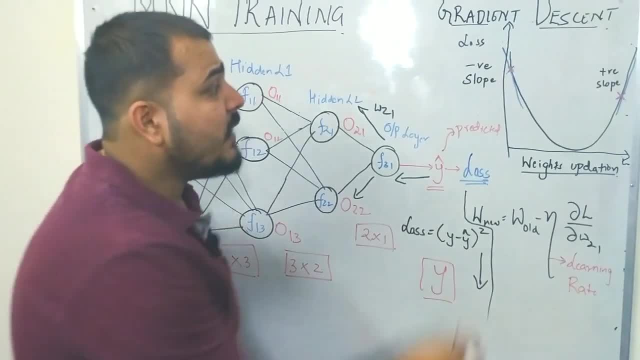 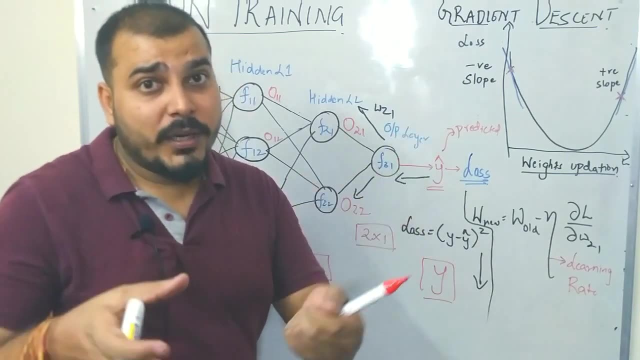 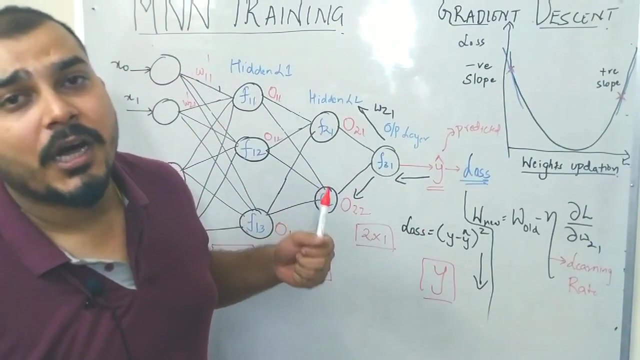 Okay, In this case it is pointing down right. Whenever it is pointing down, that basically means it is a negative slope. You just try it out. You can do it with the help of maths also, But the simple way is that whenever the right-hand side of that particular line, if it is pointing down, this becomes a negative slope. okay. 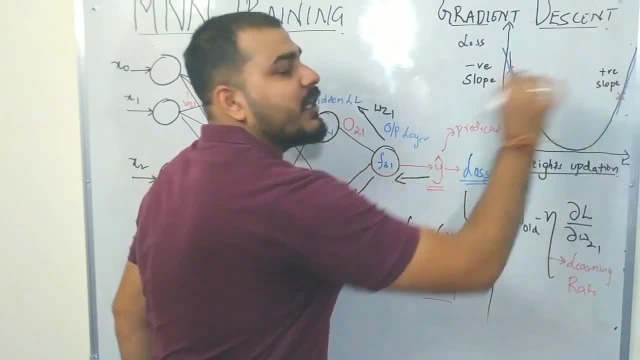 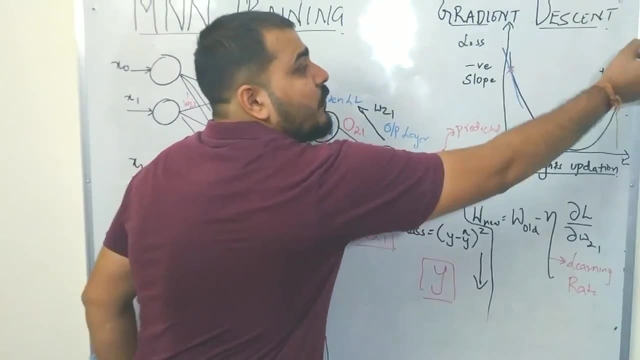 Now, similarly, let us take that the weights were initialized to this particular point. initially, I got the cost function value or the loss function value somewhere here. okay, Now I need to update the weights right Now. when I try to find out this, I try to draw a tangent line to this, to find out the slope. 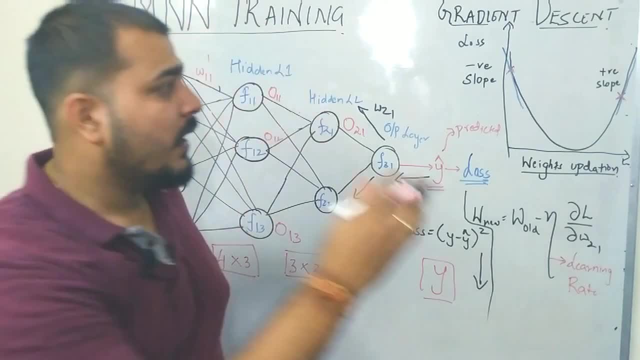 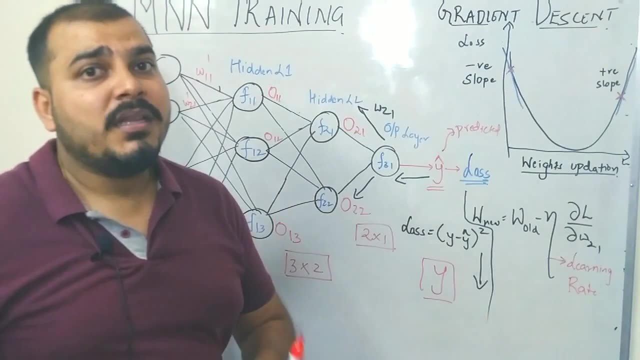 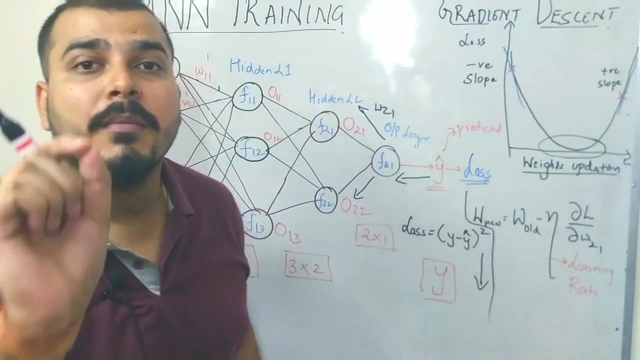 Over here. you can see that the right-hand side of the line is pointing up. It is pointing up like this: okay, This basically means that it is a positive slope. Now, always remember: the main aim of this gradient descent is that we should be reaching in this particular location, which is basically my global minima. 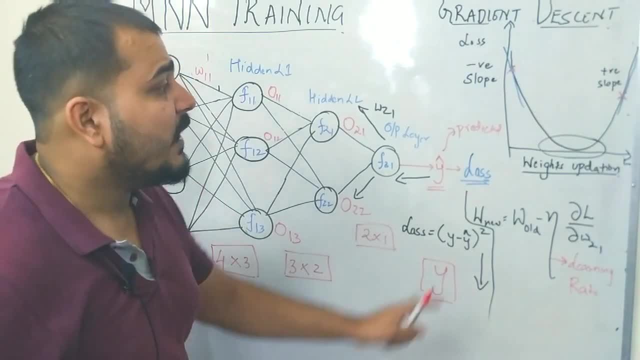 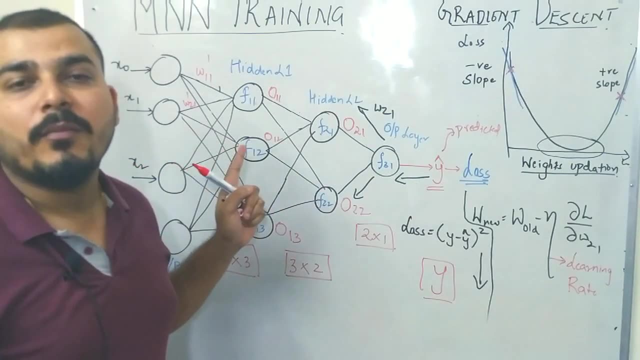 This is basically called as my global minima. And this particular global minima, unless, until you don't, Unless, until you don't Reach over here, the updation of the weights will happen with the help of back propagation. okay, And suppose if this loss value is decreasing, right? 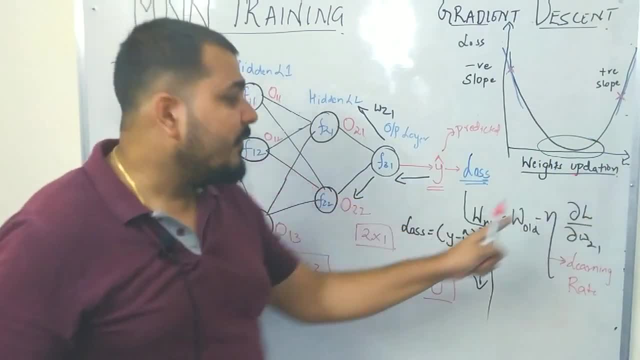 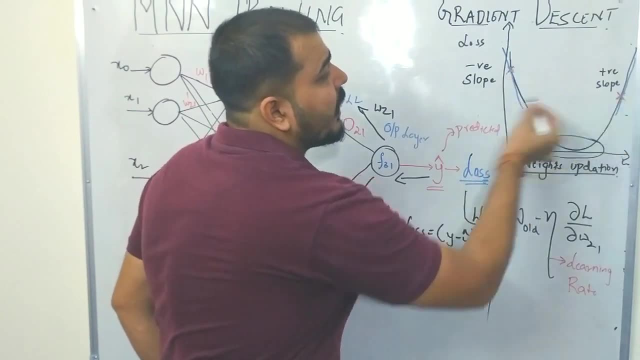 That will also indicate that we are reaching this global minima. If it is not reaching, If this loss value is not decreasing at that time, that basically means that your point is rotating here itself. okay, Now what will happen if I have a negative slope? 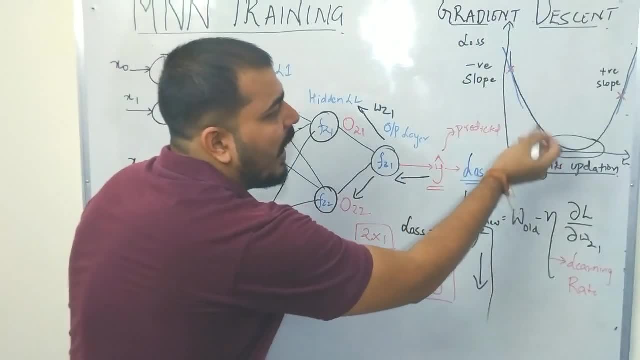 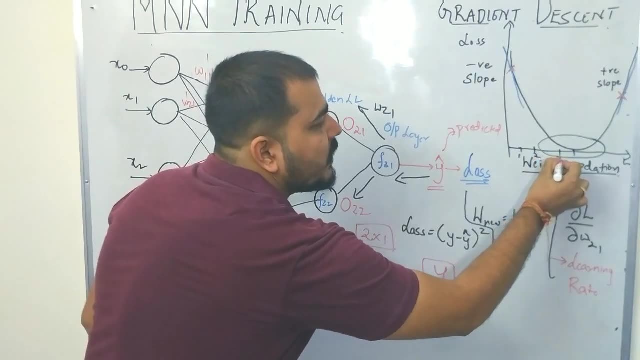 That we need to understand. okay, Suppose, if we have a negative slope, Now I have to reach over here. right Over here, my values are lower And this is a little bit higher. Suppose this is 1,, 2,, 3,, 4.. 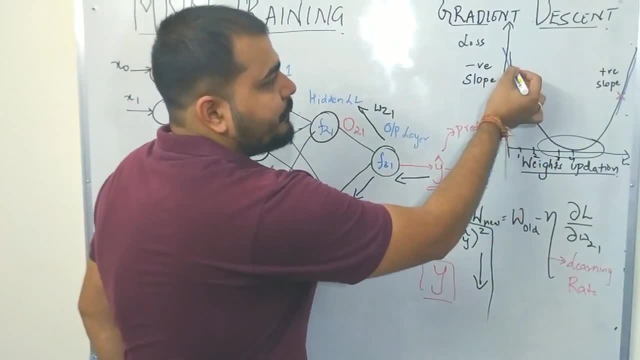 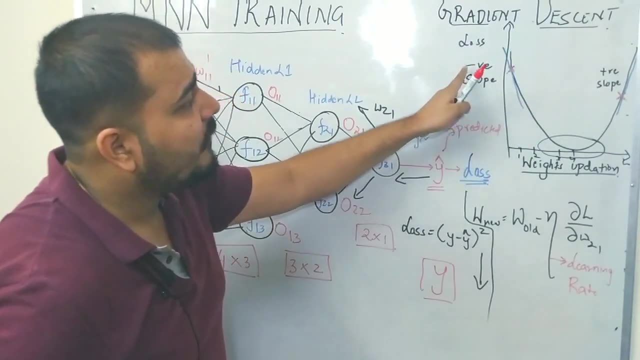 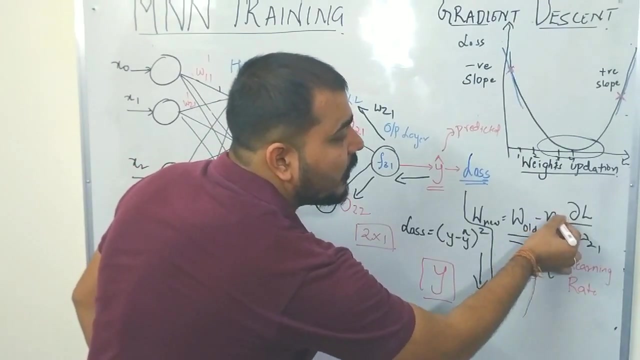 At this particular point. I have my global minima Now, initially my point is somewhere around 1.. But I have to reach at this particular point right Now. suppose for this particular slope my value is negative. Now, if my value is negative, that basically means that it will become Y-old minus learning rate, multiplied by a negative value. 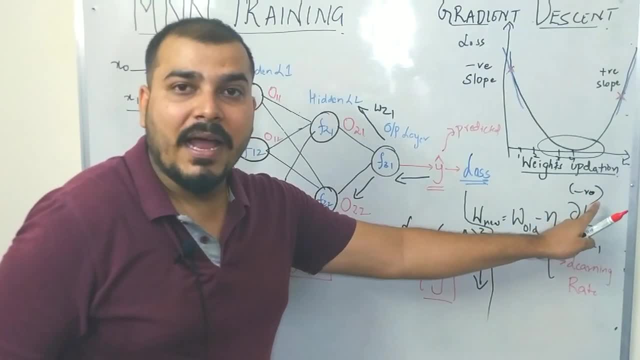 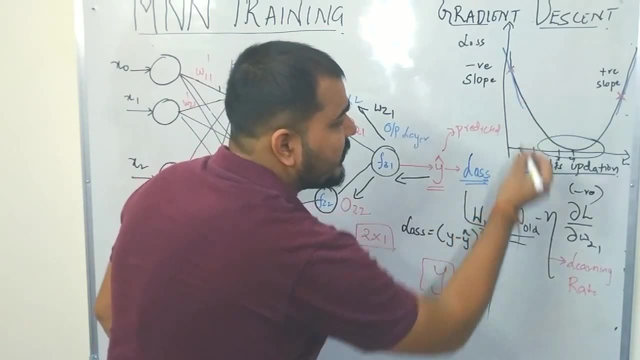 And now, when we multiply a negative value, this will become a positive value, because minus into minus is positive right Now. when it is positive, that basically means we are adding up the older weight with some value, When we are adding up some older weight with some value, right. 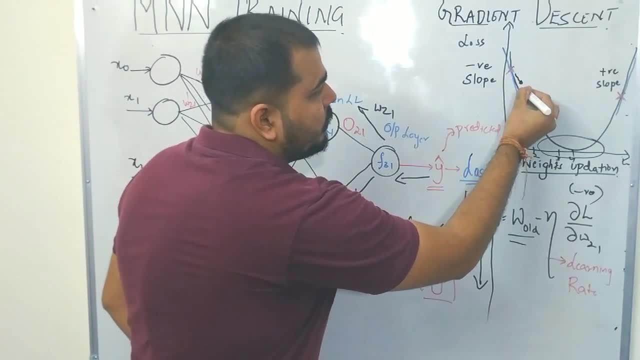 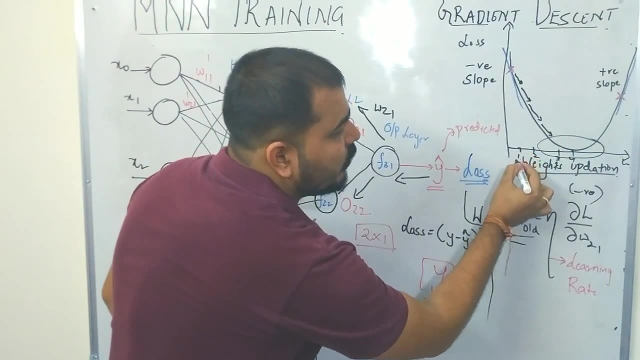 What will happen Then? the point will move down And after some time you will be seeing that. Why it is moving down? Because my initial value is 1. Now my Y-new value got increased. That basically means now it is moving in this particular direction. 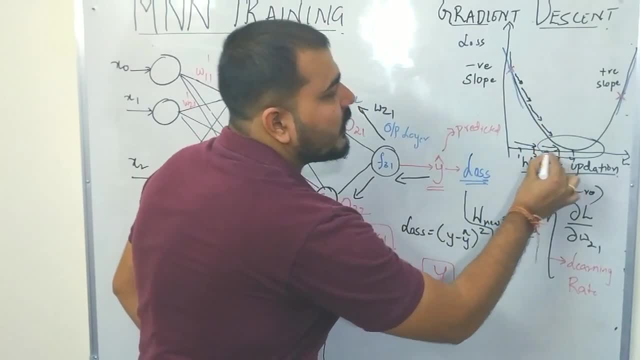 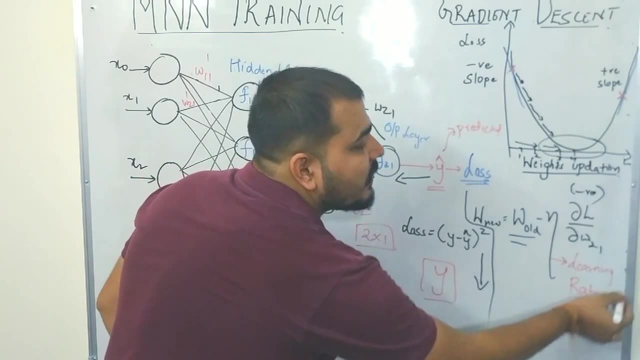 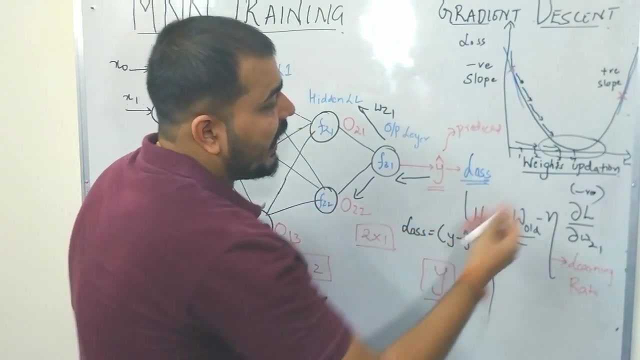 Okay, It is moving in this particular direction. right, It is moving in this particular direction. So that is how. But how slowly and how fast it should move is basically decided by this learning rate. Now suppose if I take a small learning rate value, that basically means this will take much time to reach at this particular global minima point? very slowly. 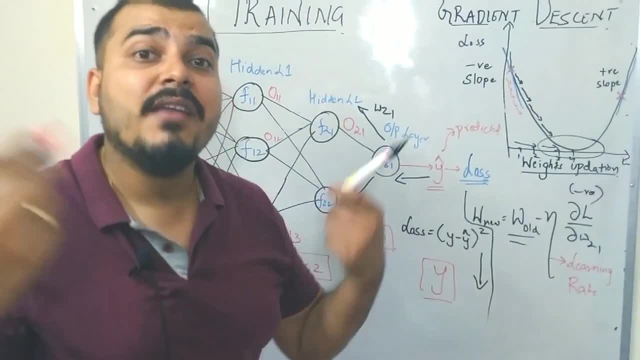 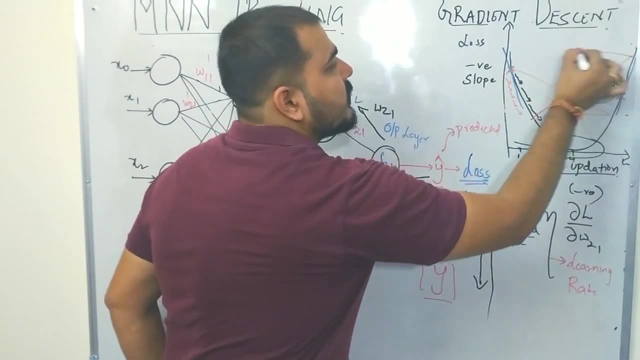 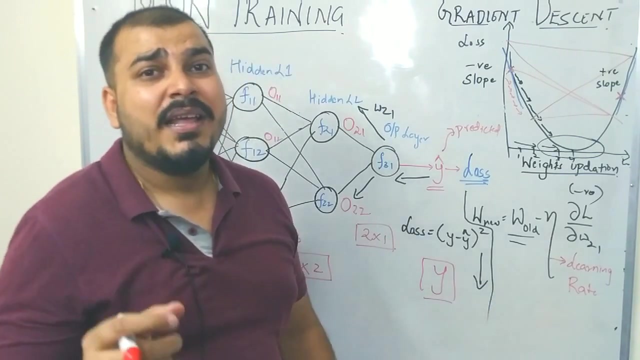 It will reach very slowly. But what happens? if we take a higher value, Very, very higher value, Then this particular weight will be jumping here and there. It will jump like this And it may never reach the global minima point. So it is always said that you should select a learning rate in such a way that it should be a value which is suitable with respect to this gradient descent. 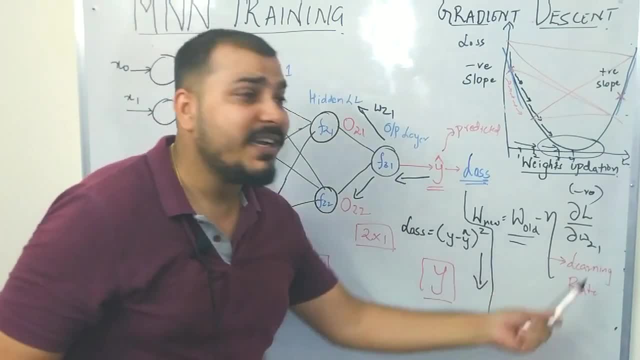 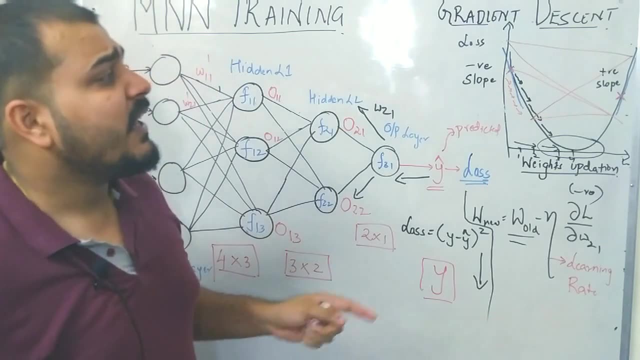 I will be helping you out how we can select a learning rate. We have to perform some hyperparameter optimization. When I will be doing the practical application, that will make sense. Now. just let me take an example of a positive slope Suppose for this particular point. I have a positive slope. 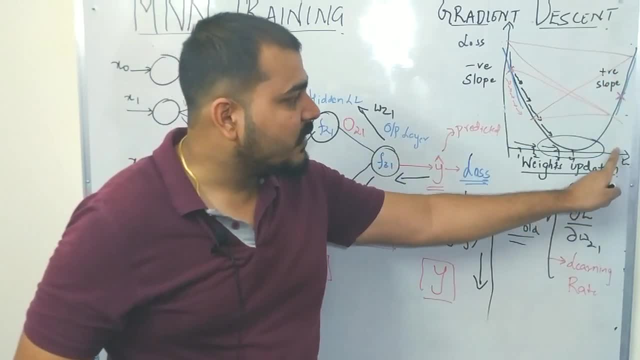 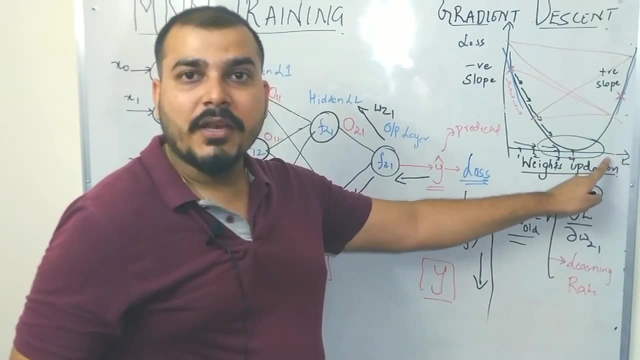 Okay Now, in this case my positive slope. if I go and see my value, it is somewhere here. But I have to reach somewhere here, Right? So I have to subtract this cost value or the cost function value, Right? 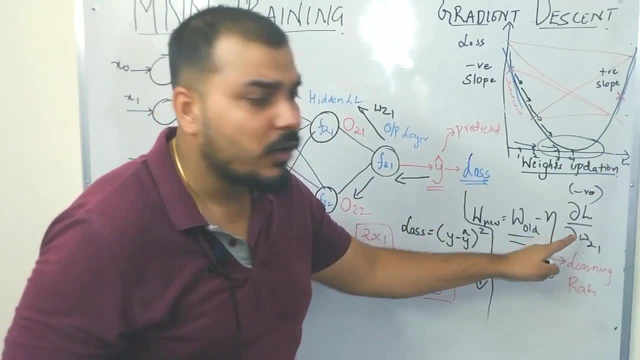 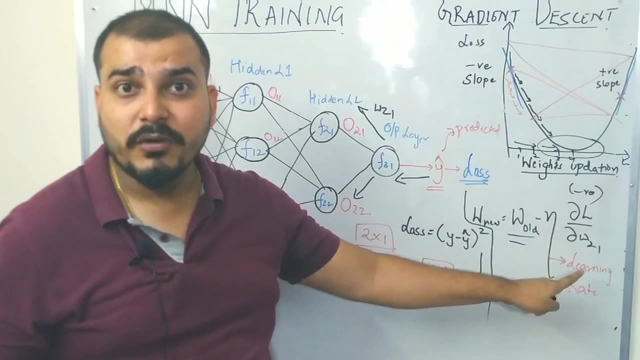 I have to subtract it. In order to subtract it, suppose let me just give my mind the same formula I have w old, minus the learning rate multiplied by derivative of the loss with respect to that weight. Okay, Now here I know that derivative is a positive value. 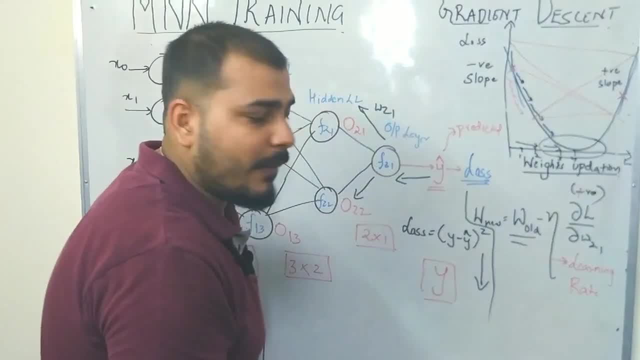 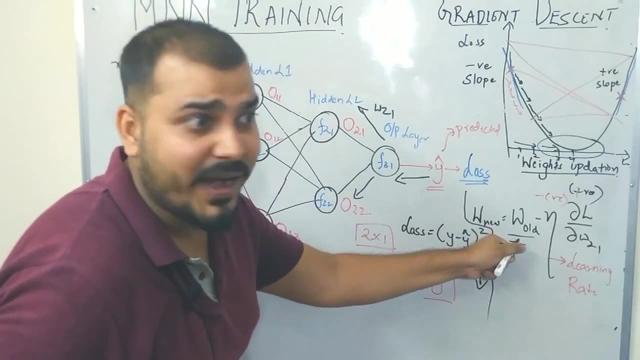 Now, when I have a positive value, what will happen? Minus into positive is a negative value. That basically means we are subtracting the old. We are subtracting the old weight with some value. That basically means my value will reduce. 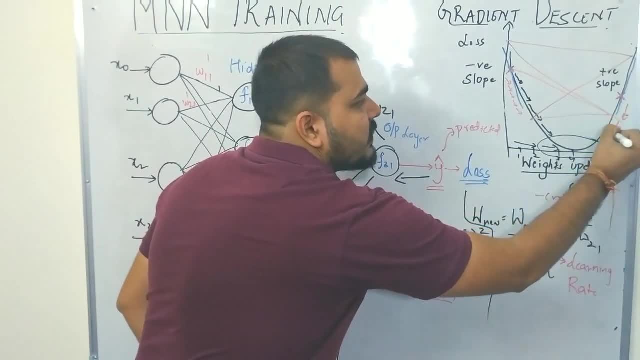 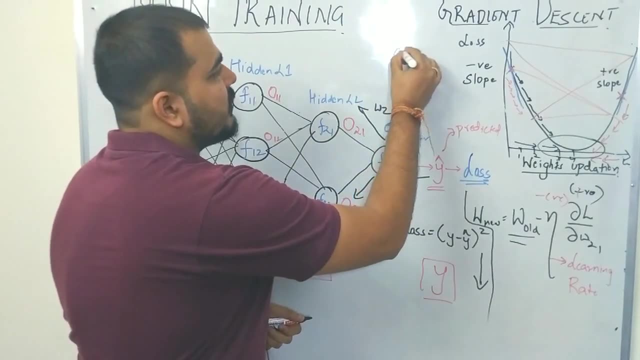 And again, how speed we have to come down, that is decided by our learning rate. So always do not select a very, very larger value. It should be some minimal value. Usually, in most of the scenarios, I select 0.001.. 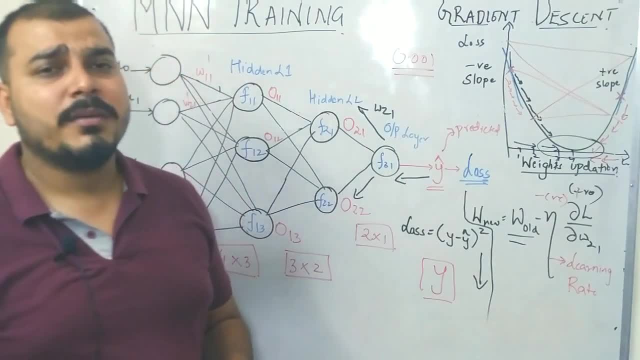 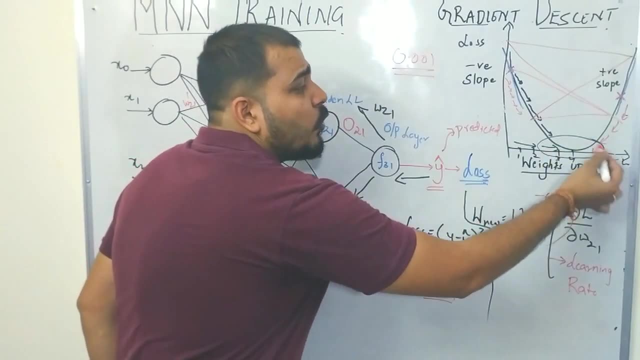 How do I come into this particular value? I do some hyperparameter optimization with respect to most of the data, But again, I will show you this with the help of practical example. Now, unless and until we do not reach this step, the back propagation will be going on. 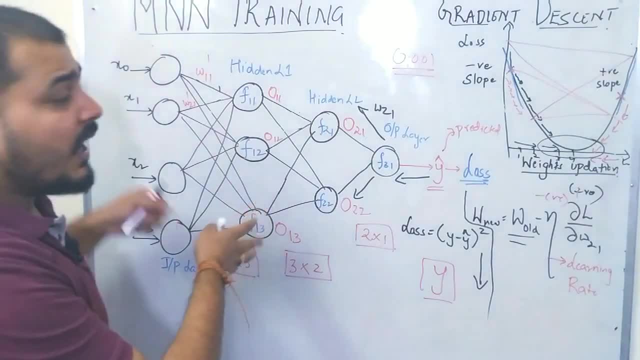 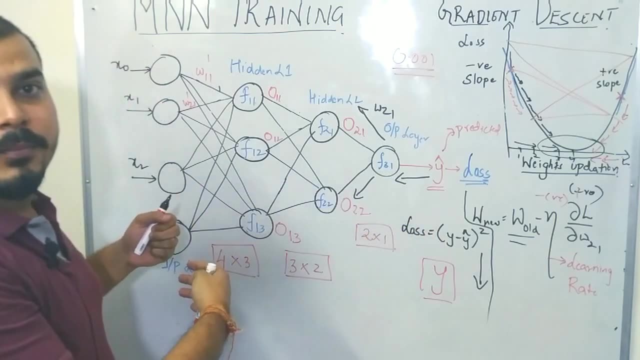 It will be updating the steps, It will be updating the weights, And then again the front propagation will be going on And again it will be updating the weights. Okay, So front and back propagation, that actually helps you to get, I mean one. 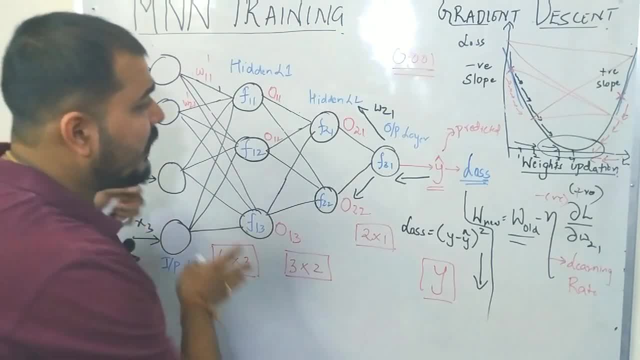 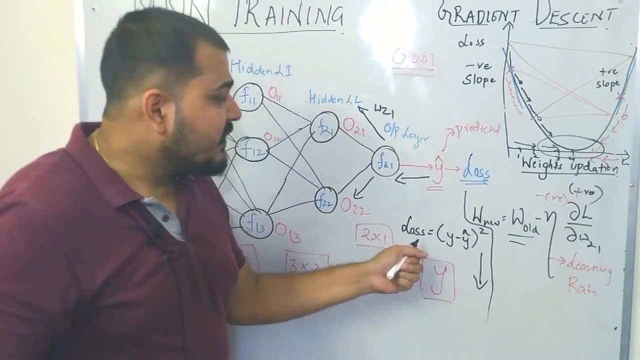 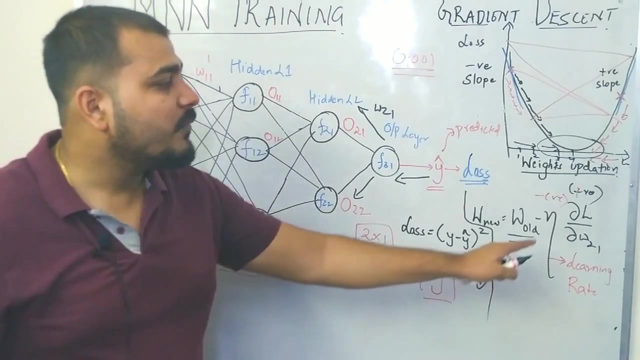 It is basically like one epoch: Okay Now. similarly, how do you know whether you are going in the right way? by selecting the correct learning rate, You will be seeing that after some epochs right, this loss value will be decreased. If it is not decreasing, guys, that basically means there is some problem with this learning rate of this particular derivative. 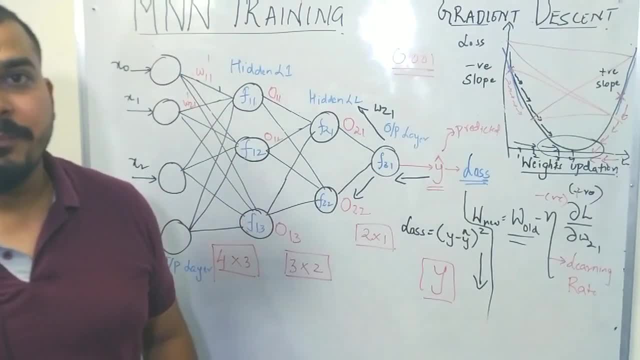 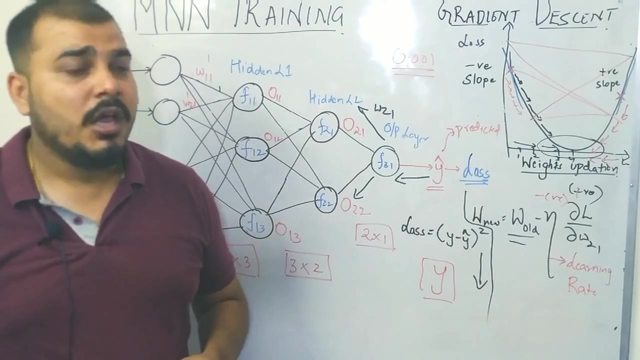 Okay, That basically means the whole function is not converging somewhere, And this is how a gradient descent works. Gradient descent works for the whole number of records. Okay, I will also be discussing about stochastic gradient descent in my next video. So in my next video I will also be discussing about something called as chain rule. 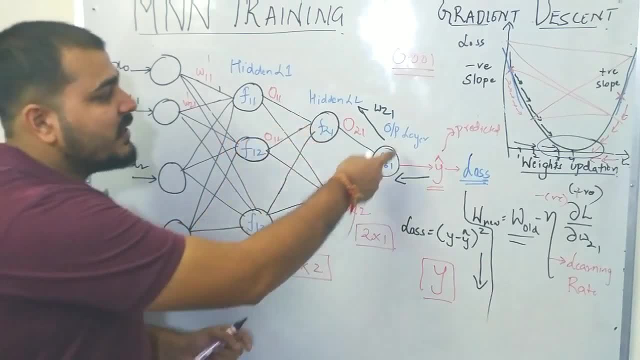 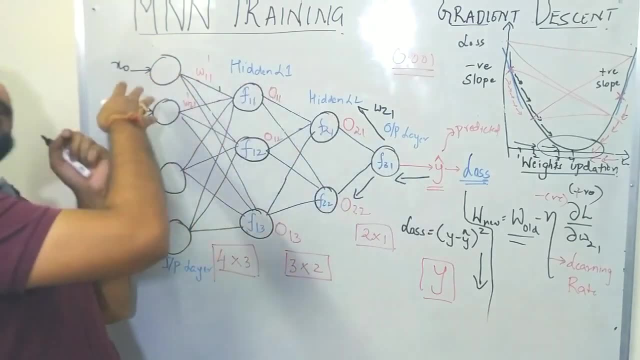 That involves a lot of maths. how the weights gets updated, Okay, How these weights will get impacted by these weights, Right? Or this weight will also get impacted by this weight. So how that chain rule will be going ahead, I will be explaining you all in the next video. 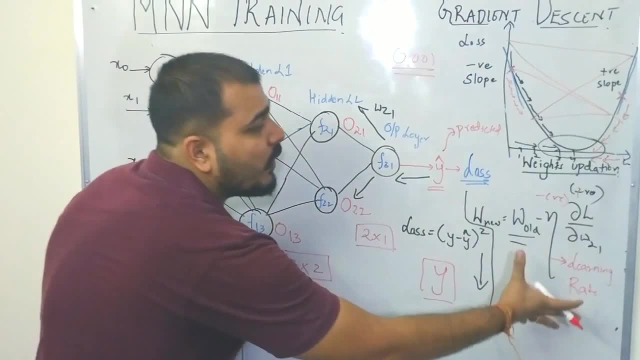 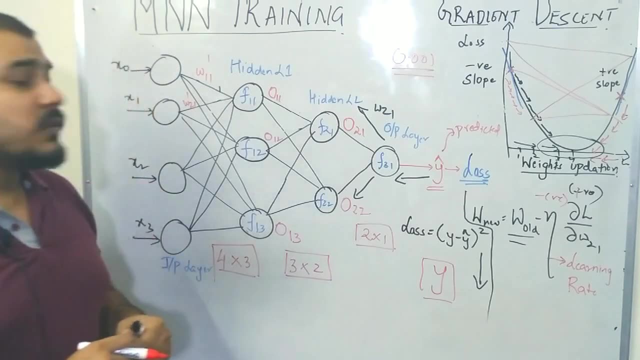 But I hope you understood gradient descent, I hope you understood this particular weight updation formula And I hope you understood a multilayer neural network, how it gets trained. Okay, So that was all about this particular video, guys. I hope you liked this particular video. 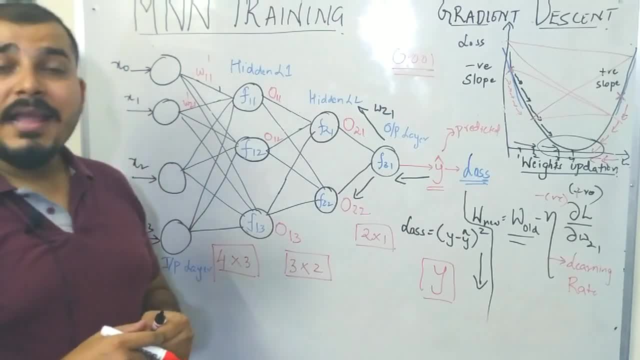 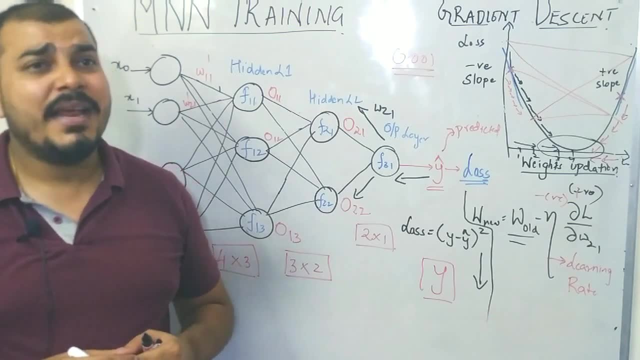 Make sure you subscribe the channel. And, yes, if you have any queries, please do comment in the comment box itself. I will come up with all the solutions as soon as possible And I will be uploading more number of videos as I go ahead. Thank you one and all. I will see you all in the next video. God bless you all.